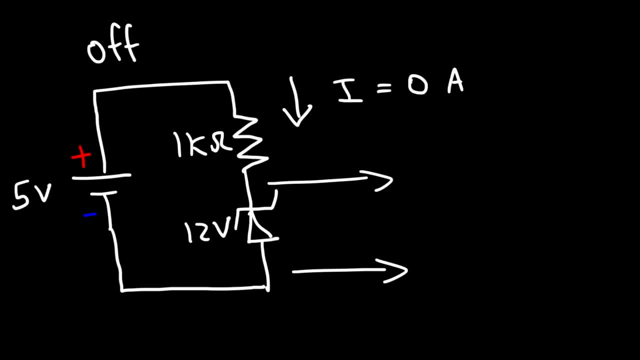 voltmeter across the Zener diode. what voltage will it read? Now, because there's no current flowing in the circuit, the voltage across the resistor is 0 volts. So therefore, the voltage across the Zener diode that will be picked up by a 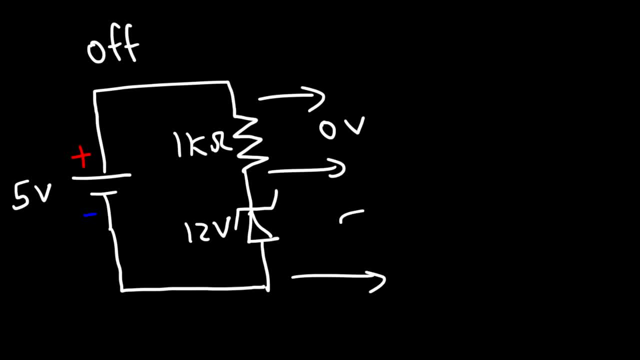 voltmeter will be the same as the voltage of the battery. It will be 5 volts, because these two they have to add up to 5.. So now let's use the same circuit, but this time we're going to increase the voltage of the battery. 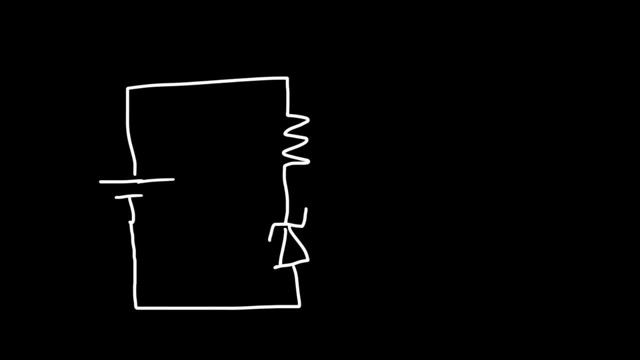 so let's make it, in this case, 14 volts instead of 12 or 5. now is the circuit on or is it off, because the input voltage exceeds the reverse breakdown voltage of the zener diode. the circuit is going to be on, and so there's going to be a. 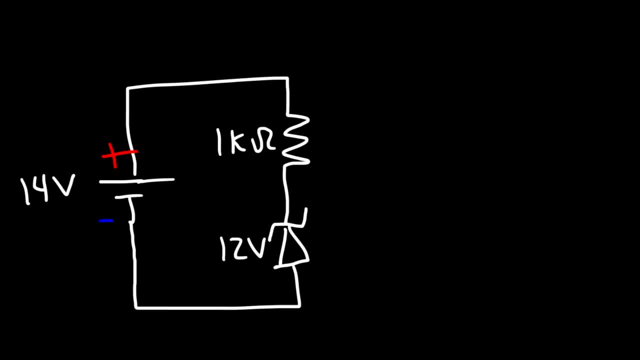 current flowing through this resistor. so how can we calculate the current in this circuit? how can we find the answer? in order to find the answer, it's important to understand that the zener diode serves as a voltage regulator, so as long as the current is around, basically the characteristic current for this, 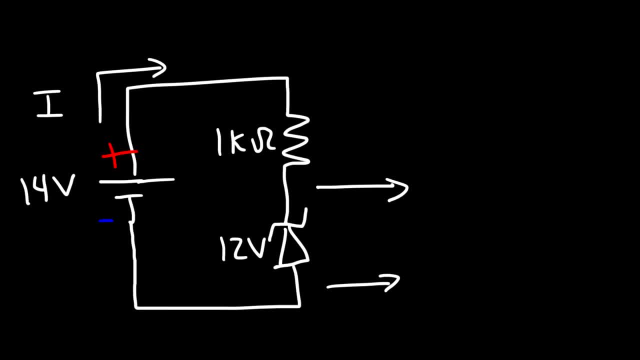 particular zener diode. let's say, if it's small, it's not too large. the voltage across the zener diode will remain approximately 12. it might vary a little, but for the most part, for all practical purposes, we're going to say that it's about 12. it could be 11.9, 12.1, but it's going to be fairly constant. so 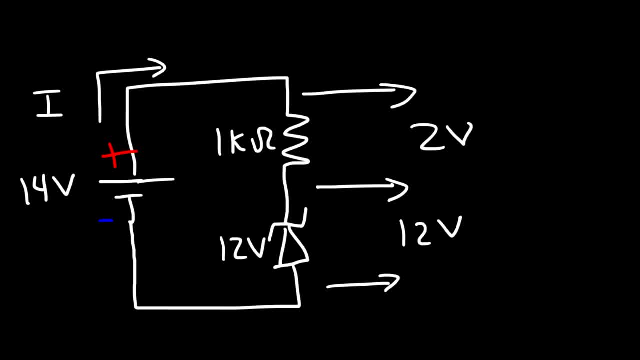 that means that the voltage across the resistor has to be 2 volts, because these two they have to add up to the voltage of the battery. so we have 2 volts across a 1 kilo ohm resistor. so if we use V equals IR, then 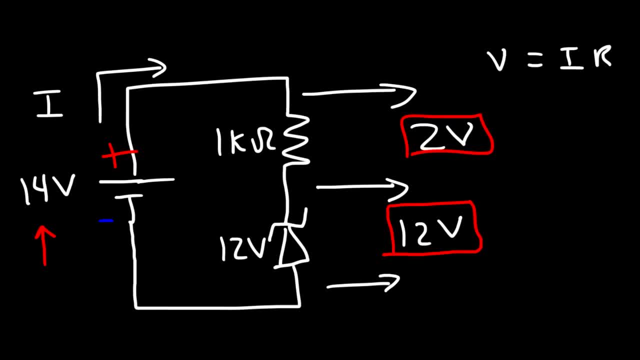 the voltage, while the current flowing through that resistor is going to be the voltage divided by the resistance, so it's going to be 2 volts divided by a thousand ohms, which is going to be .002 amps or 2 milliamps. so that's the 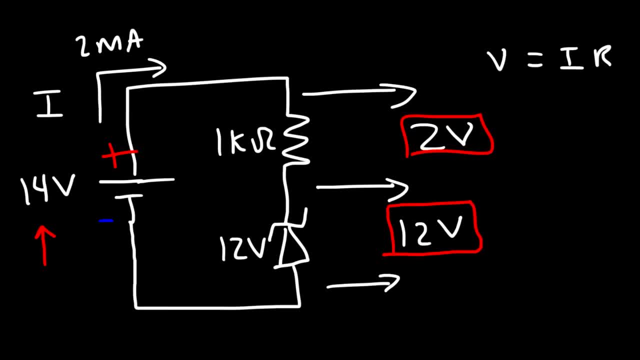 current that's flowing in this circuit. but it's important to understand that the zener diode will maintain a relatively constant voltage of 12 volts when it's in reverse bias mode and if the input voltage exceeds that value. that is the rating of the zener diode. now let's 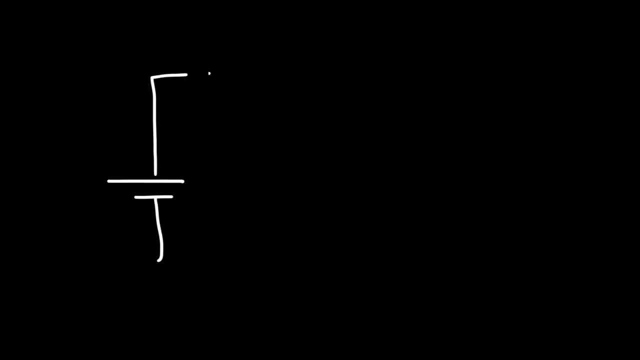 increase the voltage of the battery. so let's use the same circuit with the same components. so we have a 12 volt zener diode, but this time let's use a 50 volt battery. so what is the voltage across the zener diode and what's going to be the current? 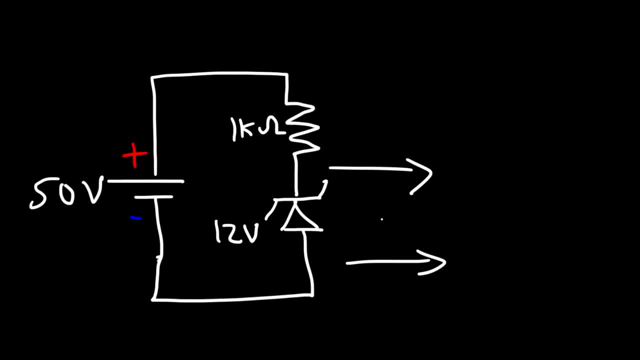 in the circuit. in this case, the voltage across the zener diode will still be approximately 12 volts, which means the voltage across the resistor has to be 50 minus 12 or 38 volts. so if we take 38 volts divided by 1 kilo ohm, 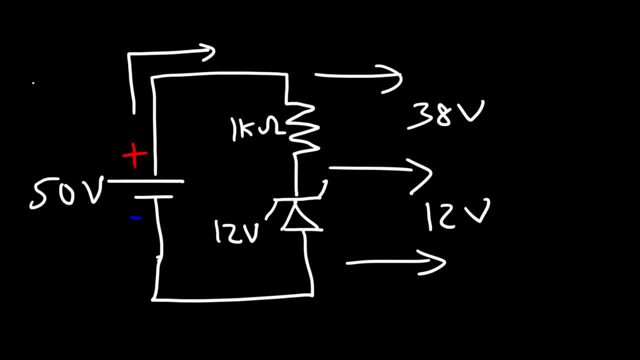 that will give us a current of 38 milliamps flowing through that resistor and through the entire circuit. so that's how you can easily determine the current flowing in such a circuit whenever you have a resistor in series with a zener diode. now there's a lot of other stuff that we can do, so here's another circuit. let's 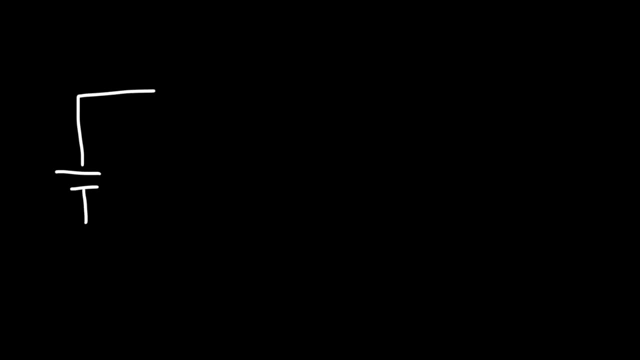 say, if we have a 50 volt battery and let's use a 1 kilo ohm resistor again, but this time we're going to use two zener diodes as opposed to one, and let's say the radian for each zener diode is 12 volts. so what is the current flowing in a circuit now? so 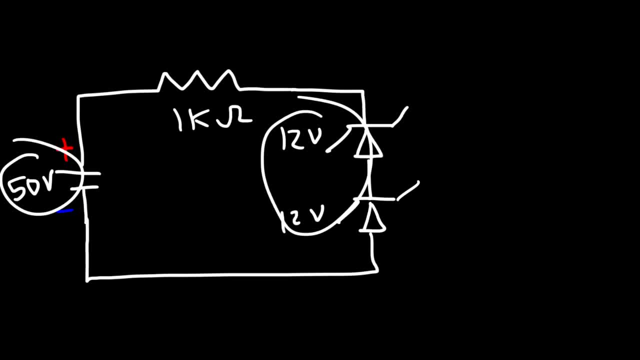 the input voltage exceeds the total reverse voltage of the two zener diodes, which means the circuit is going to be on and so the voltage drop, or the voltage across those two zener diodes is going to be 12 plus 12, so we're going to. 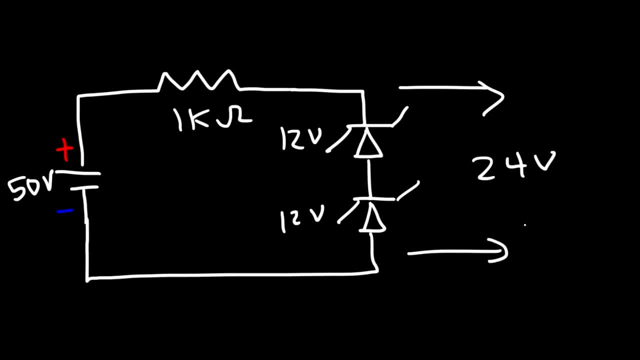 have 24 volts across those two zener diodes, which means the voltage across the 1 kilo ohm resistor is going to be 26, because 24 plus 26 adds up to 50. so if we take 26 volts and divided by a 1 kilo ohm resistor that's going to give. 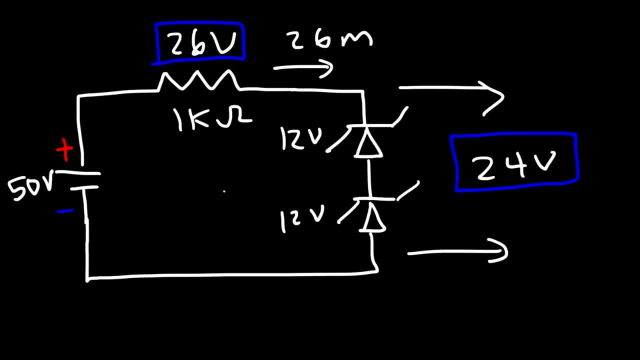 us a current of 26 milliamps flowing in this circuit. but if you want a simple way to calculate the current, it's going to be the input voltage, which is 50, and minus the total reverse voltages. of the total reverse voltage, rather, of the two. 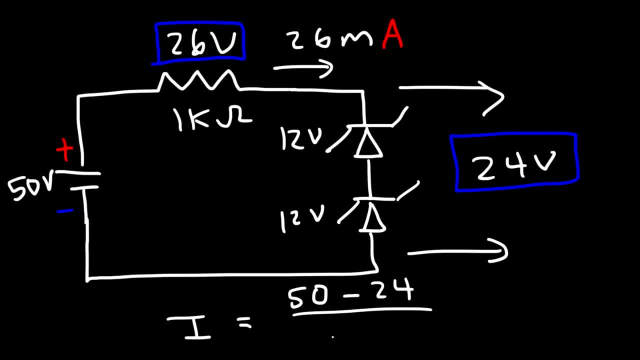 zener diodes, which is 24, and then you divide that by the 1 kilo ohm resistor, which is a thousand ohms, and so 26 divided by a thousand, that's point zero to six amps. and then you can convert that to milliamps by multiplying it by. 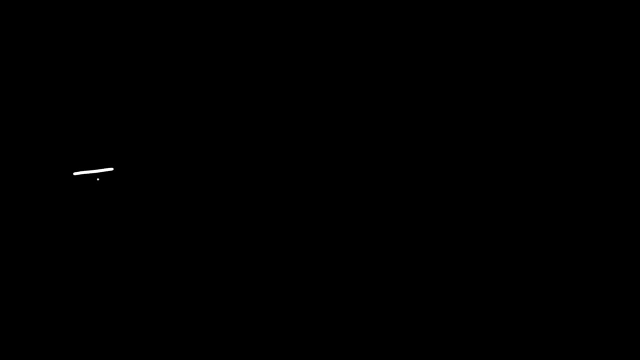 a thousand. so here is a generic formula to calculate the current in the previous circuits. it's going to be the input voltage minus the total reverse zener voltage divided by the resistance in the circuit, and so that will give you the current flowing in the circuit. now let's say if we have an AC sine wave connected. 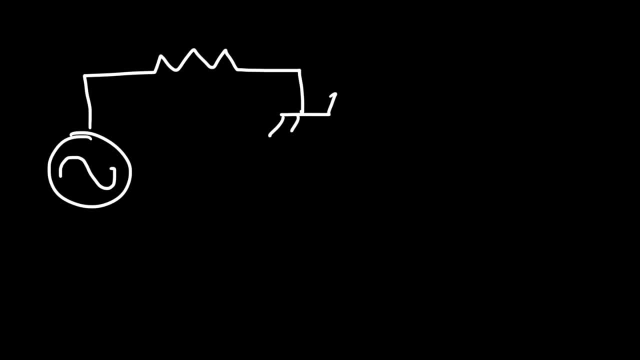 to a resistor and two zener diodes connected like this. so what's going to happen? let's call this point a, let's call this point B and then we'll call this d1 and d2. so when current is flowing in this direction, notice that d2, the arrow points in the same direction as the current. 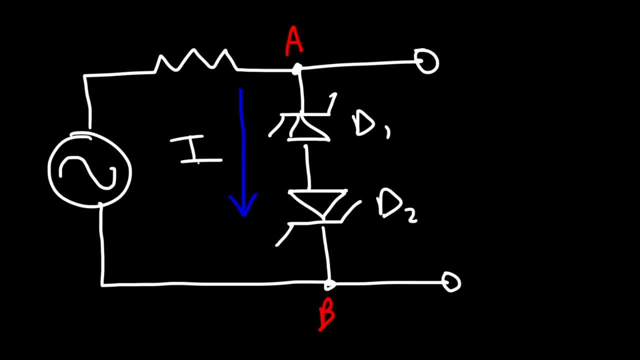 so in that case that diode will be in its forward operating mode, which means you'll have a voltage drop of approximately 0.6. and this diode it's in reverse mode because its arrow is opposite to the direction of the current, so it's voltage drop will be 12. so therefore the voltage across A and B will.